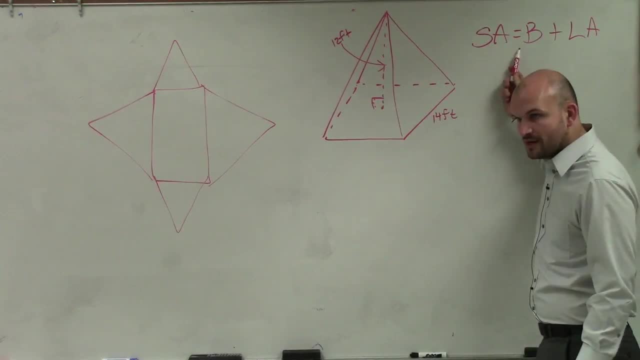 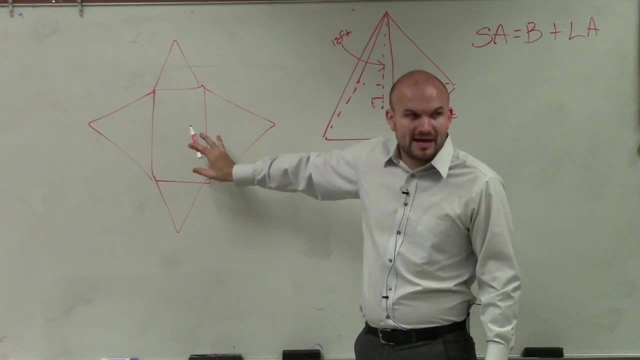 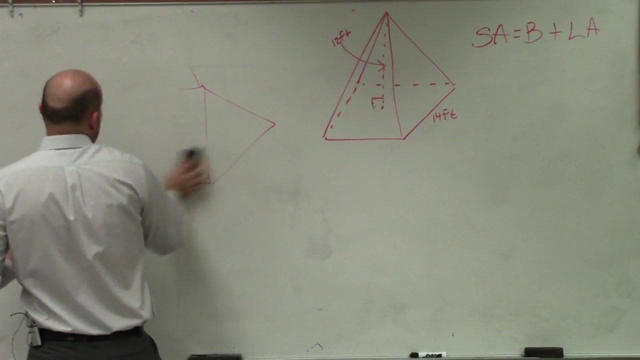 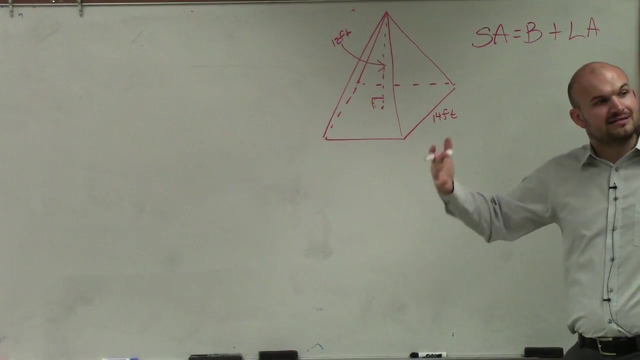 have a regular base. you cannot use this formula If you have a regular base, or the formula that I'm about to give for the lateral area. if you have an irregular base, you have to find the area of each side length and then add them all up together. But fortunately for us, we have a regular polygon as a base. So therefore, since we have a regular polygon, I just need to find the area of all those sides, So the area of the base that's regular, That's base times, height. 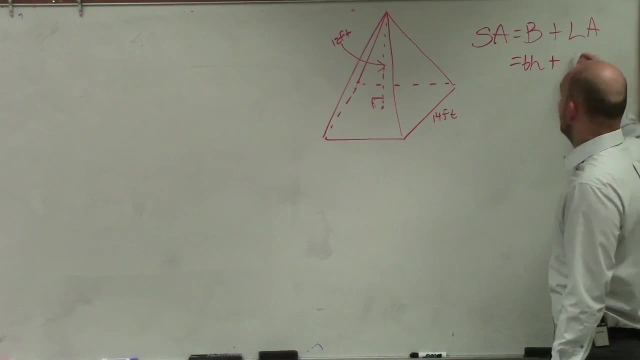 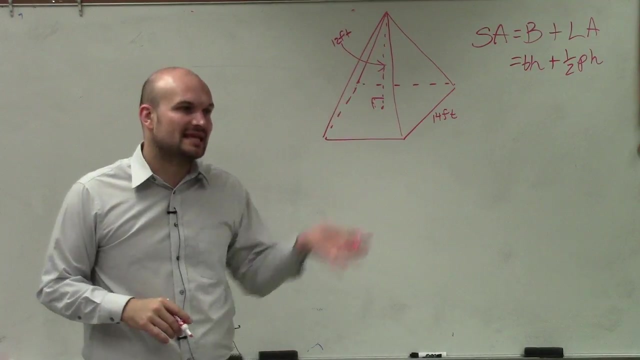 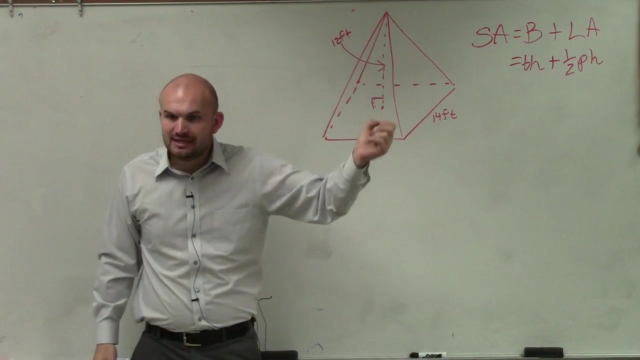 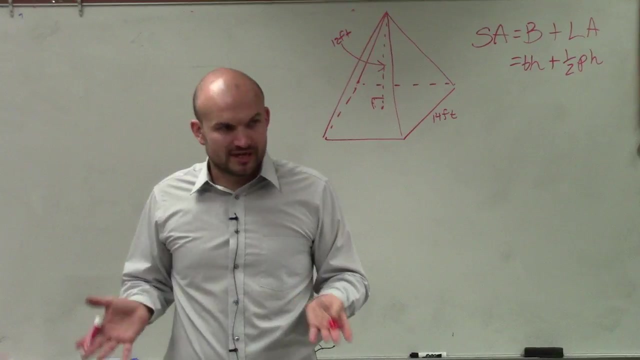 Right, Because it's a square. Plus, the lateral area is one half perimeter times H. Now, remember, H represents the slant height. What we have is the height from the bottom to the top. That's not the height we need when we're dealing with surface area. And I'm going to give you guys another little nugget to think about When you're talking about surface area, when we're talking about 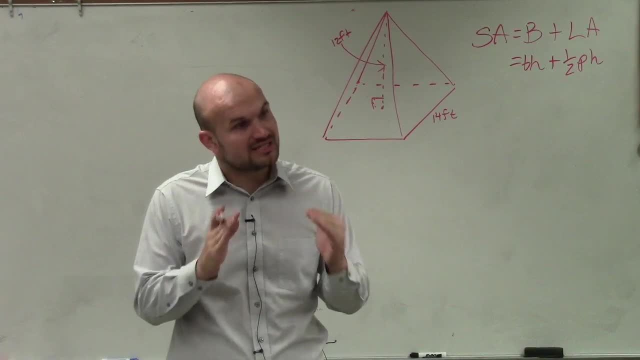 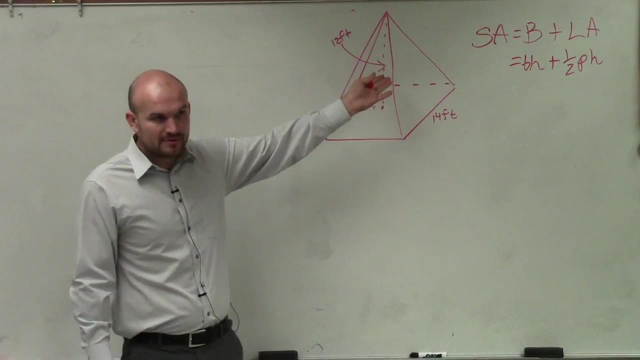 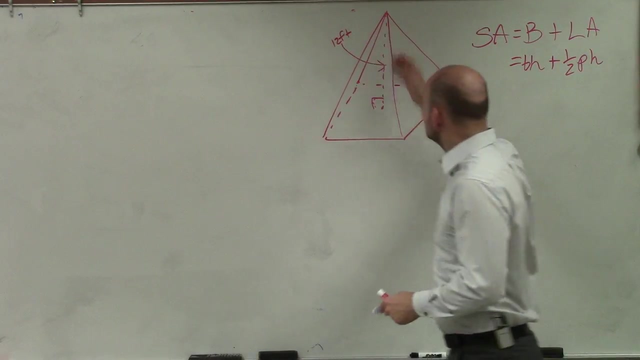 surface area and we have slants. we want to use the slant heights. When we're talking about volume, we always want to use the distance from the base to the top, But since we're talking about that, the issue we have here is we have. what we have right now is we have the distance from the base to the top. We need to find the slant height, So therefore, we need to figure out what that distance is. 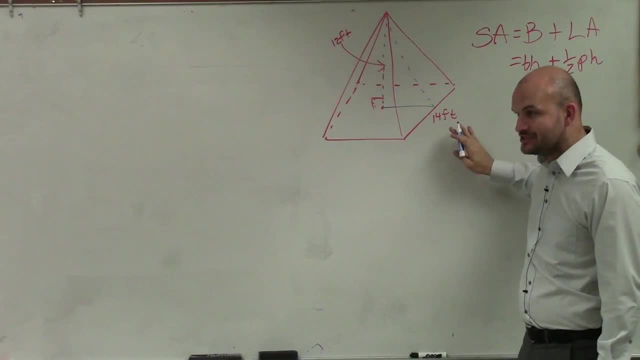 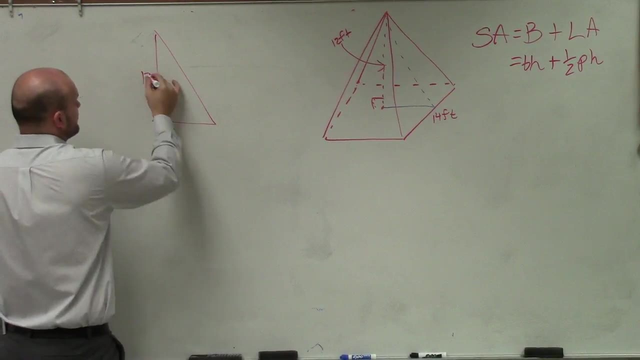 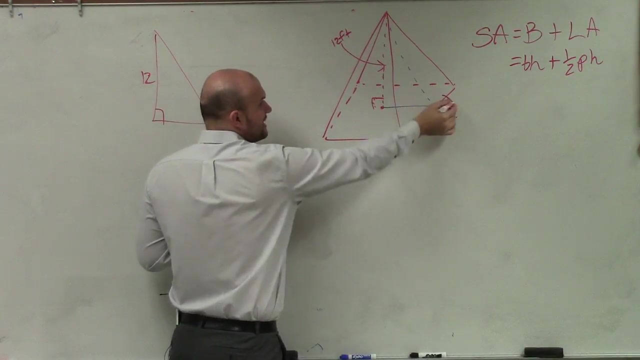 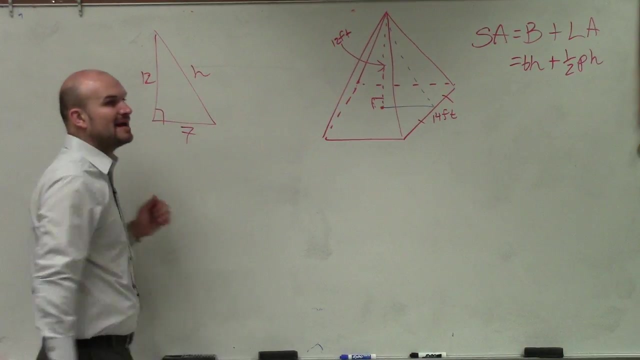 This distance from the base to the top on the edge. So therefore, I need to go ahead and look at that And I'm going to redraw the triangle. That distance is 12.. Now, ladies and gentlemen, if this comes directly down in the middle, that means that cuts this in half. So if this whole distance is 14,, that means that side of the triangle is 7.. So is it possible for me to find my H, which is the slant height I have to use? thank you. 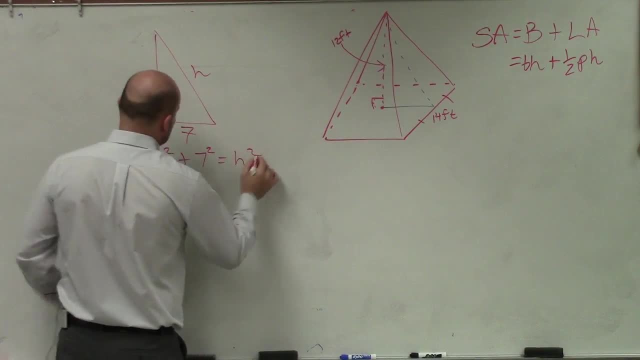 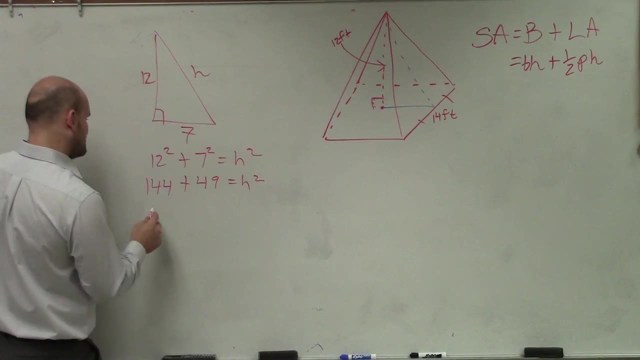 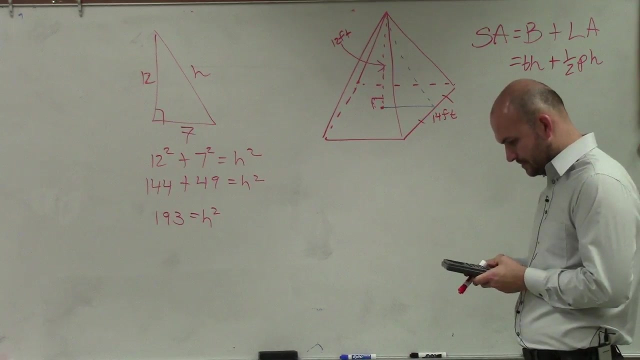 So I have 12 squared plus 7 squared equals H squared. 12 squared is 144 plus 7 squared is 49, equals H squared 80, so that's 193.. So I have 193 equals H squared. So now I need to take the square root of 193.. I'm going to get 13.89..